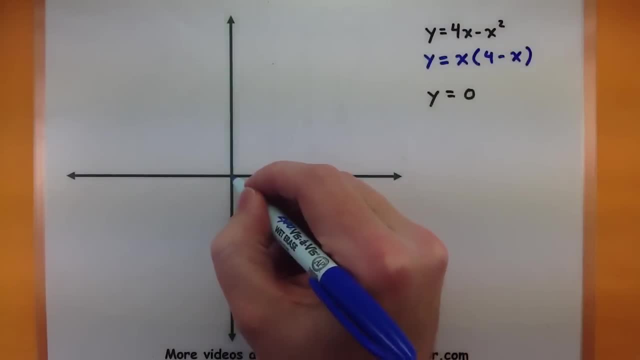 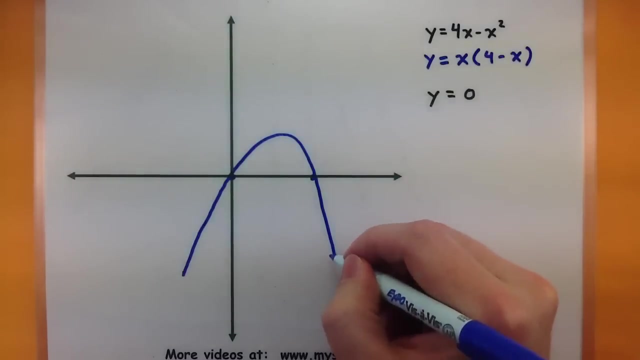 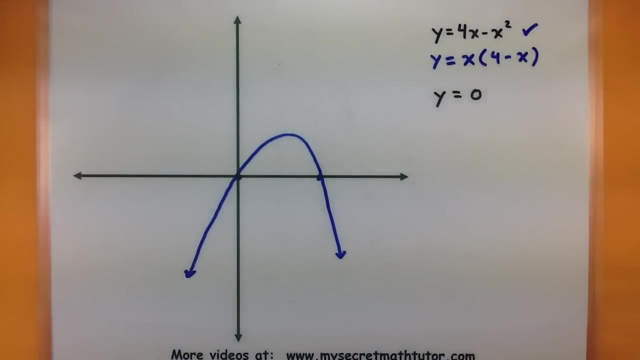 this parabola is that it crosses when x equals 0 and when x equals 4.. So this parabola looks something like this: goes through x equals 0, turns around and through x equals 4.. Now the other line that it's bounded by is y equals 0. And you should recognize that. 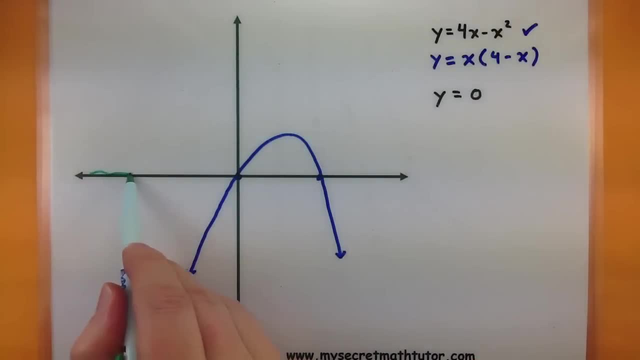 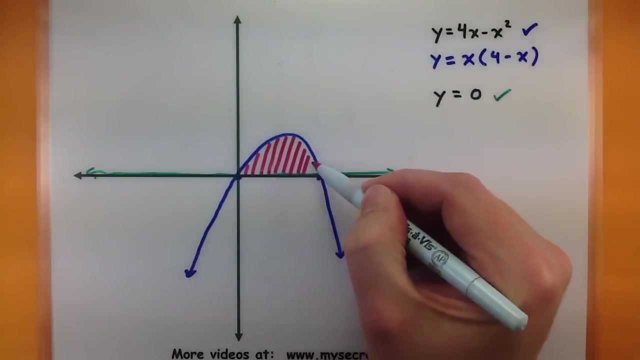 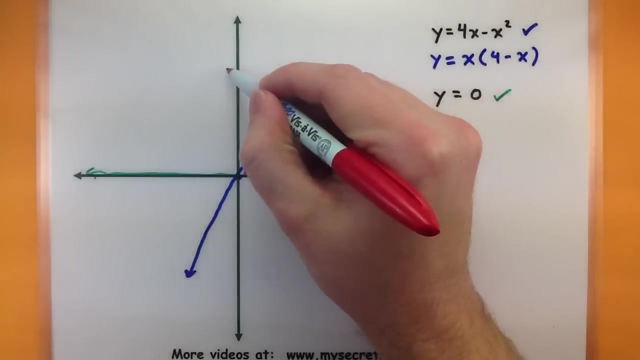 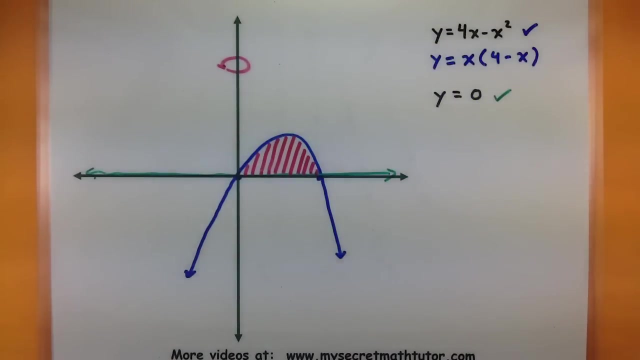 as a nice horizontal line, Just like this. y equals 0. So the region we're talking about is this little curved region right in here. Now, what makes this problem interesting is that we are going to rotate this about the y axis. Now, because we are rotating this about the y axis, we run into some interesting problems. 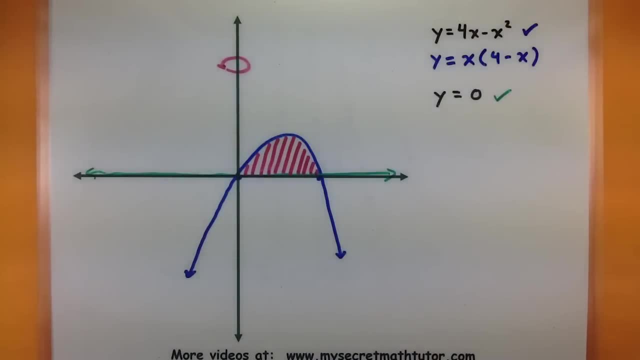 Normally, when going through a rotation problem, we can usually take care of these using, say, circular cross sections. But that's not going to be quite as easy with this guy. If we say, rotate it around the y axis like this and look at the cross sections, they do look. 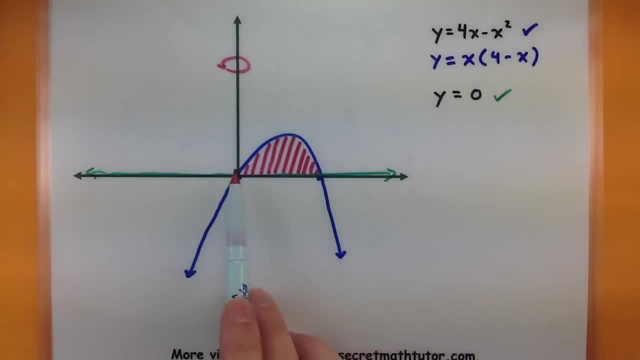 like circles. however, there's only one function that would determine, say, the inner radius and the outer radius. So instead, we're going to approach this a different way, known as the shell method. The way this works is that, instead of looking at circular slices, we'll look at shells, which 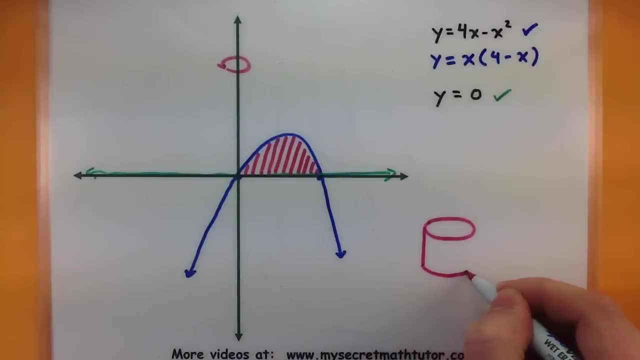 are essentially the shape of cylinders And you can imagine a whole bunch of these cylinders stacked up around one another so that they form the object. So things like this, Some things you want to know about this cylinder is that when we're talking about it, we can 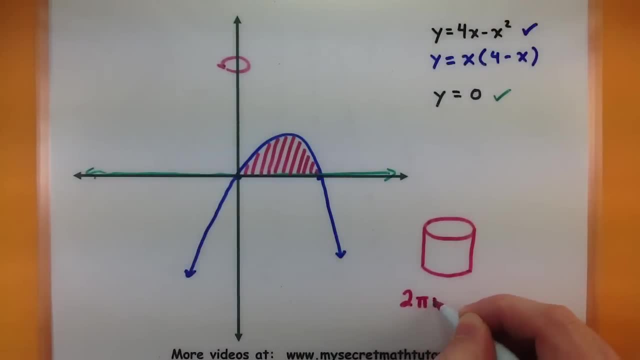 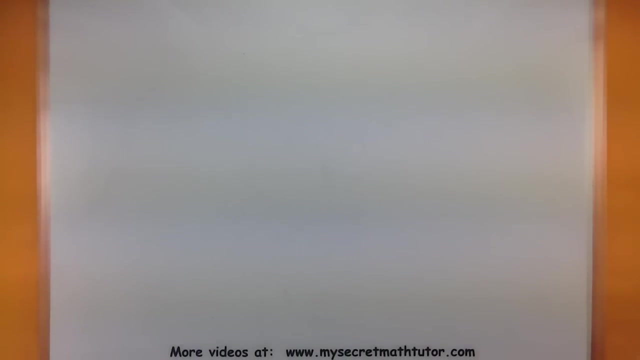 figure it out using 2 times pi, times the radius, times the height. Alright, let's go ahead and build our integral and take care of this volume, Alright. so, in general, when working with the cylindrical shells, We're going to set up our integral from a to b. 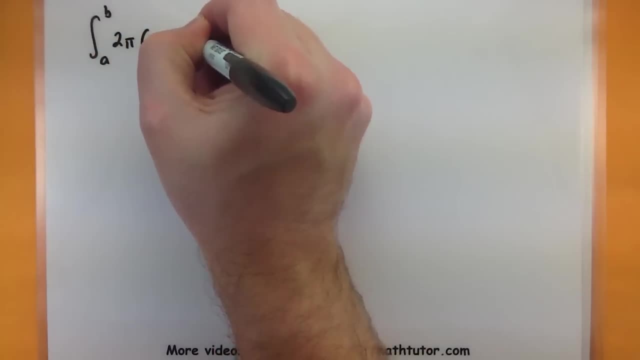 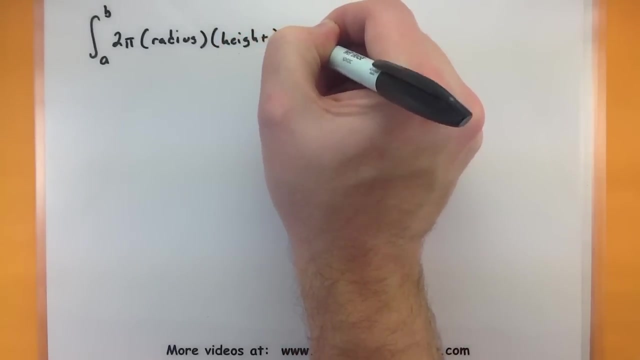 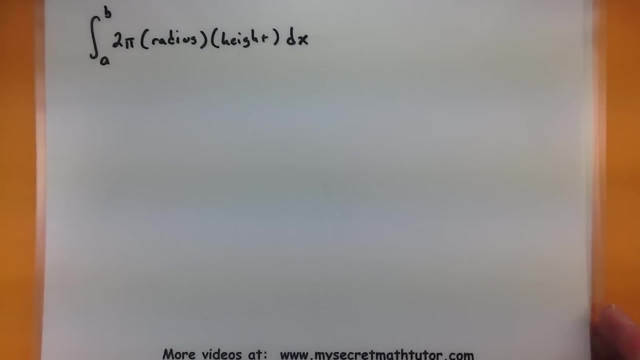 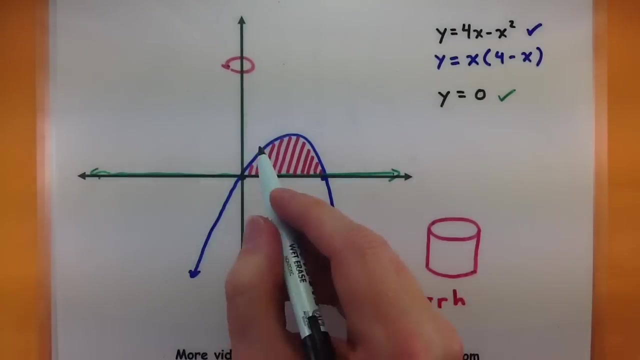 2 pi, our radius, Our height, And I will take this with respect to x. Right now, looking at our diagram, let's see if we can figure out what the radius and the height are going to be. So this is being rotated about the y axis. 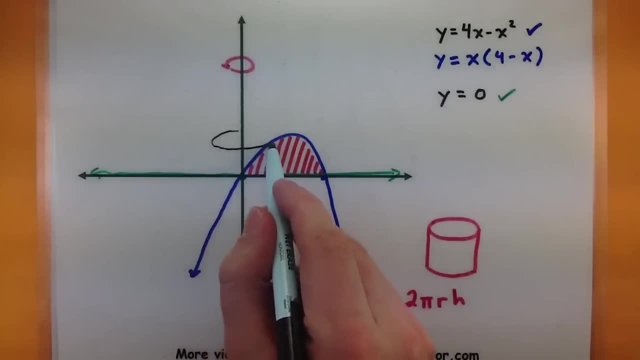 Which means that if I look at the diagram, I'm going to have an integral from a to b. look at a particular say shell in here. say, right, like that. we can see that the radius of this shell is really determined by where we are on x and the height is really being. 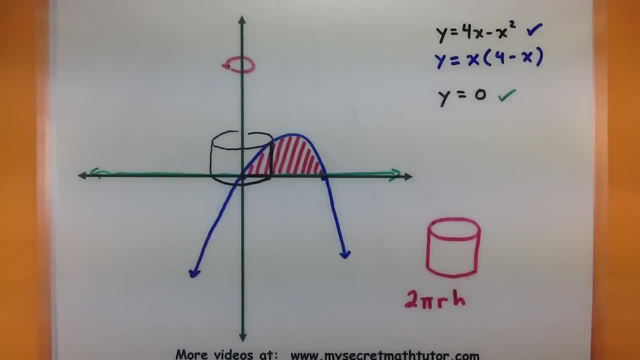 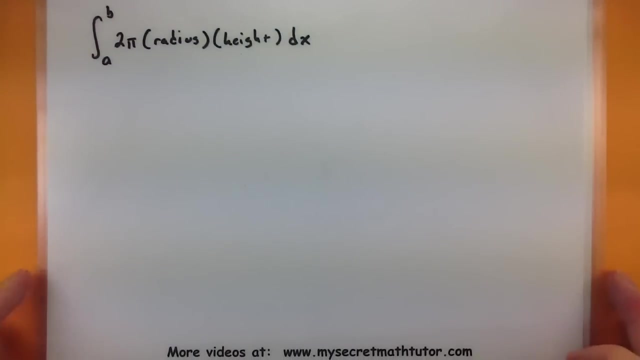 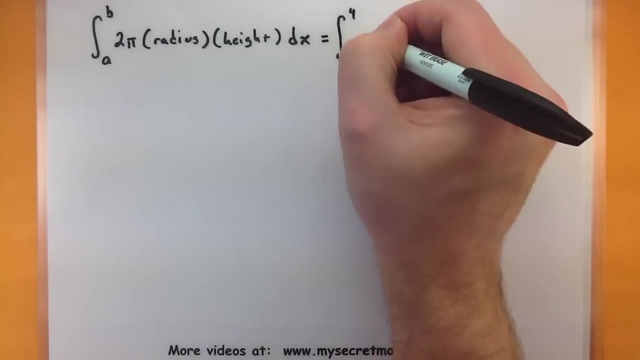 determined by the function itself. So we'll put both those pieces in so that our integral is good. Also, our radius will move all the way from 0 to 4.. So those will become our bounds. So our more general form will now look like: from 0 to 4, 2 pi times x and 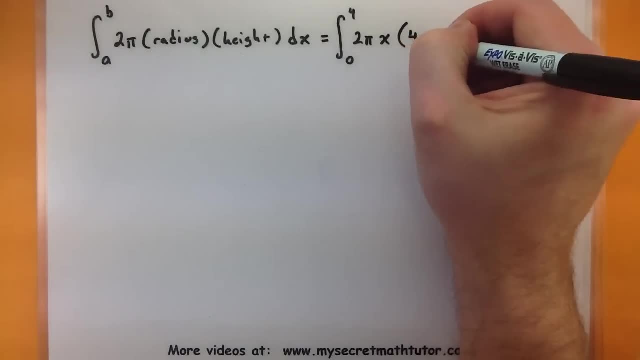 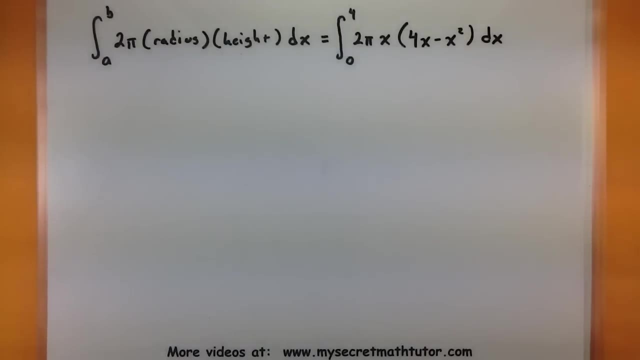 here's where our function goes in: 4x minus an x squared dx. All right, Well, now that we have everything in, we want to work on finding the antiderivative and computing from that. Like all integrals, be sure to take out any constants of integration first, And I'm also. 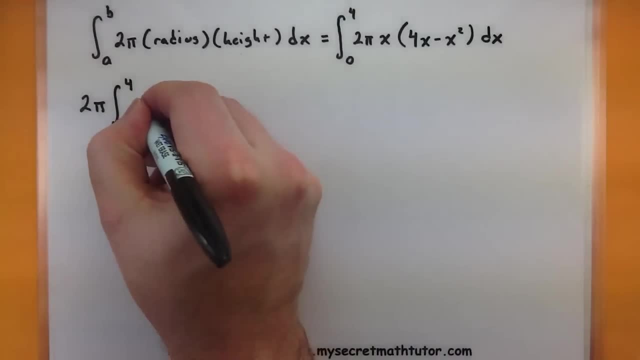 going to distribute my x into parentheses. Here's a 4x squared minus an x cubed. All right, Now that we have that, we'll go ahead and take the antiderivative of this polynomial. So add 1 to the power. 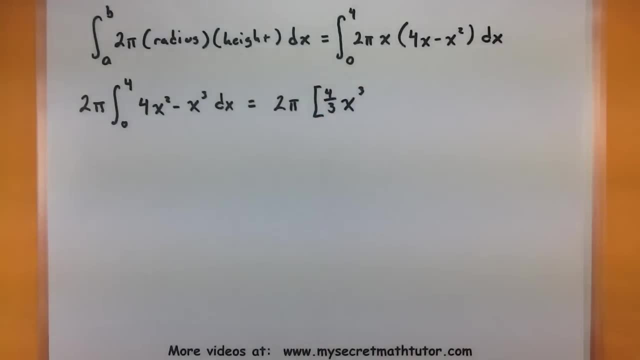 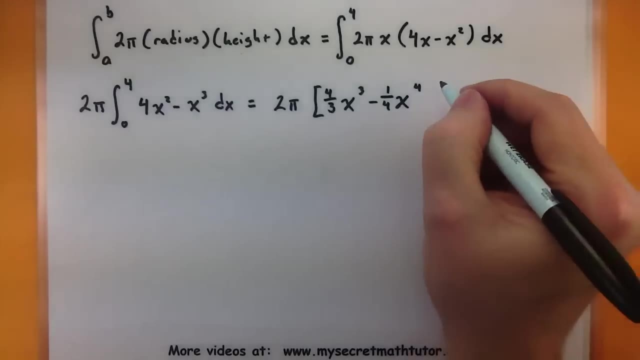 So 4x cubed And divide by that new power, so 4 thirds Minus. Add 1 to this power, Divide by that new power And evaluate it from 4 to 0.. Looking good, OK, Plugging in. 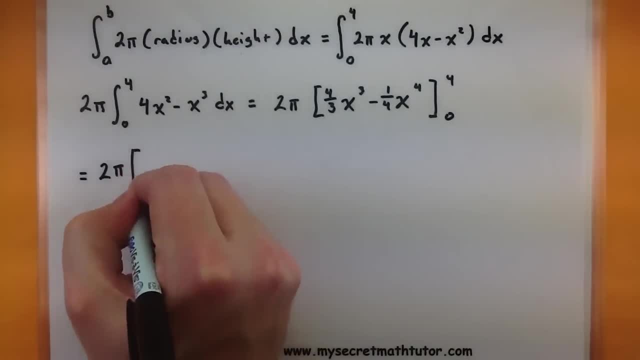 our top bound and bottom bound, we'll get just a step closer to what our answer actually is. So: 4 thirds. 4 to the third Minus, 1 fourth. 4 to the third Minus: 1 fourth Minus. 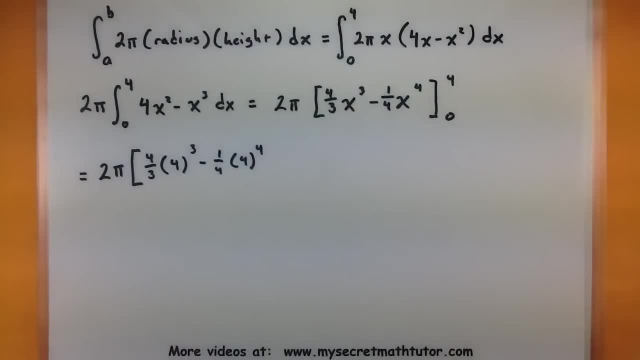 1 fourth, 4 to the fourth, And it looks like when we plug in 0,, both these guys will also be 0. But I'm going to write those out just so you can see. So there'll be a 4 thirds. 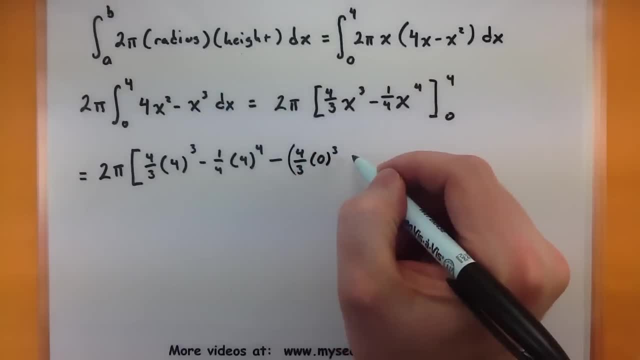 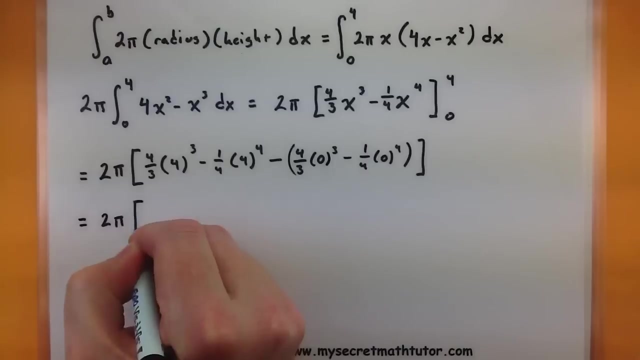 0 cubed And let's see There'll also be a 1 fourth, 0 to the fourth. Again, those guys will be 0, but just so we keep track of everything. All right Time to simplify this down. So I'm looking at 4 to the third power, which 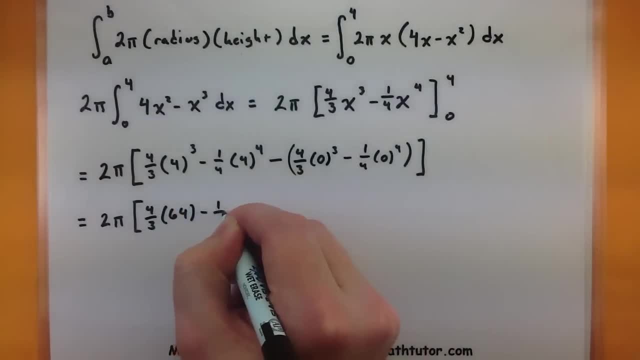 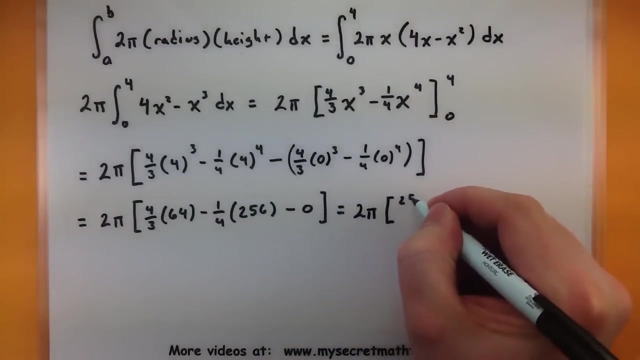 will give us a 64.. Meanwhile, a 4 to the fourth power do 56.. And, of course, minus 0.. With these guys we can start combining them with our fractions: 64 times 4 thirds, So 256 all over 3.. Minus 256, all over 4.. There we go. Now we want. 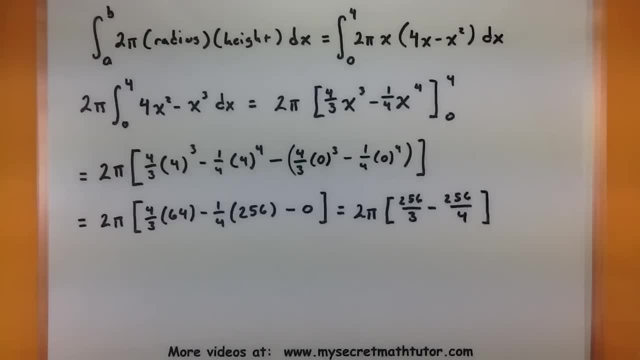 this in the simplest form. So let's go ahead and work to get those fractions together, combine them with our 2 pi, and then we'll reduce as much as possible. So a common denominator in our case would be a 12,, which means I'll multiply this one And then we'll get a 12.. 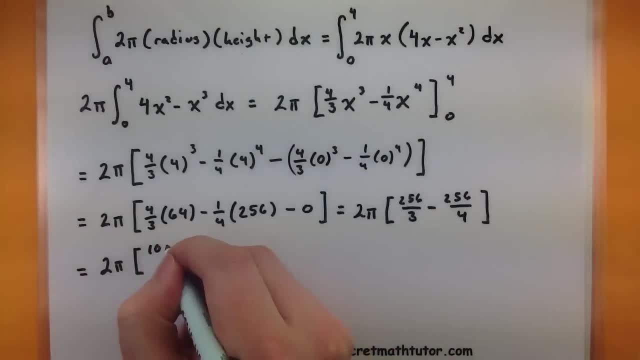 one by 4 and this one by 3.. This will give us a 1024 all over 12, minus a 768 all over 12.. Perfect. So, taking 1024 minus 768,, this will give us a 256 all over 12.. Now that's. 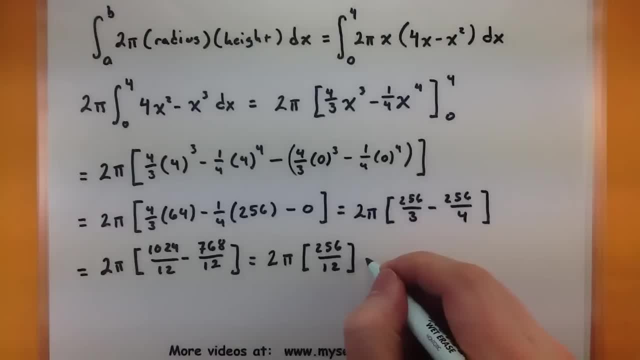 a really good fraction. It actually reduces by quite a bit. This will be 2 pi, Let's see. and then I have 64 divided by 3.. All right, I think we can finally combine that with our 2 pi in the front and get our final answer. So the volume of this guy is equal to 128 pi all over.